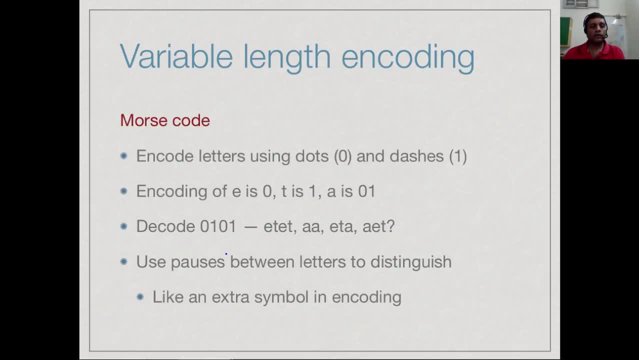 Morse assigned them codes of a dot that is 0 for E and a dash that is 1 for T. Then Morse picked other frequent letters, such as A, and gave them two letter encoding. So A is encoded, A is encoded as dot dash or 0, 1.. Now the problem with Morse's encoding is that it is 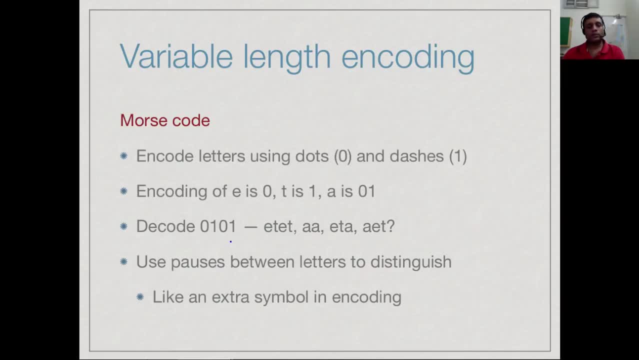 ambiguous when you come to decoding. So, for instance, if we look at the word, the sequence 0, 1, then we do not know whether we should interpret each of these as a one letter code and get E T E T or, for instance, we should think of this as two, two letter codes and 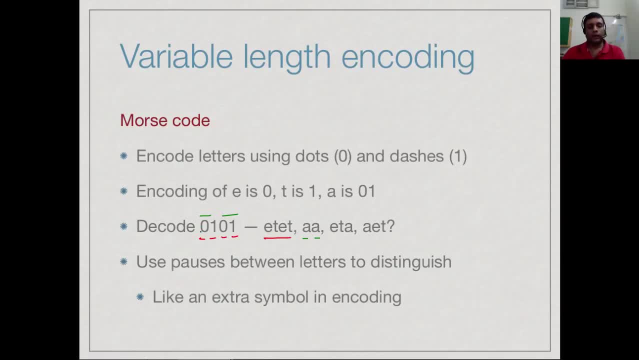 get A, A and so on, right. So depending on whether we stop at a 0 or change 0 to 0- 1, we can get many different interpretations. Now, in practice, in Morse code, what used to happen is that the operator gives a slight pause indicating the end of 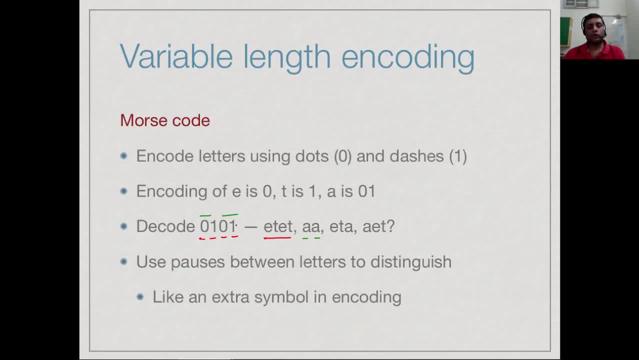 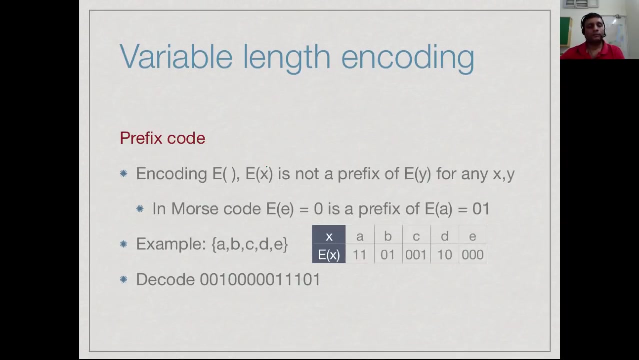 the letter. So therefore, effectively, Morse code is not a binary code, but it is a three letter code: 0, 1 and pause. Now, when we are using, of course, digital computers, we do not want to go to 3 letters, So we want to efficiently do this using just two letters. So, in order, 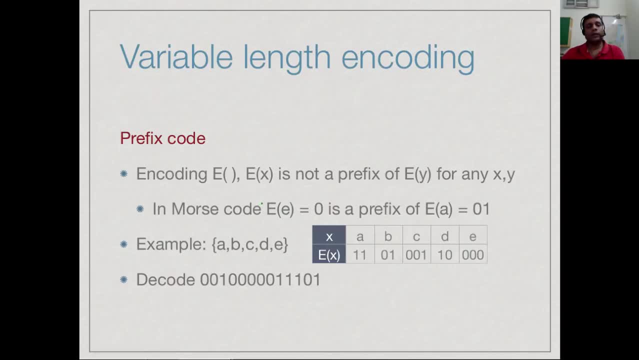 to make a variable length code and unambiguously decodable, we need what is called the prefix property. ok, When we read through a sequence of 0s and 1s, we should be unambiguously clear whether we have read a letter or there is more to read. We should not be like the earlier. 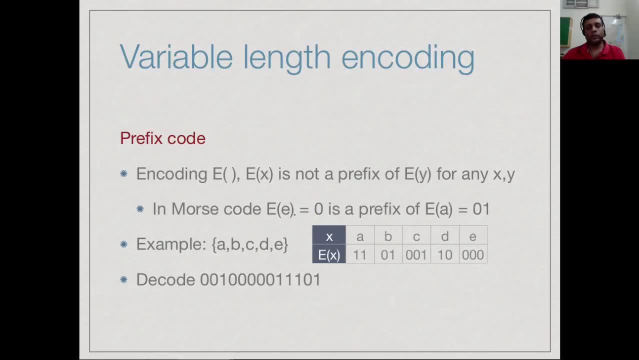 case where we have read 0 and we do not know whether we stop at 0 and call it an E in the Morse code setting, or we want to call it an A, which is a 0, 1.. So we are going to use this capital letter E to denote the encoding function. So E of. 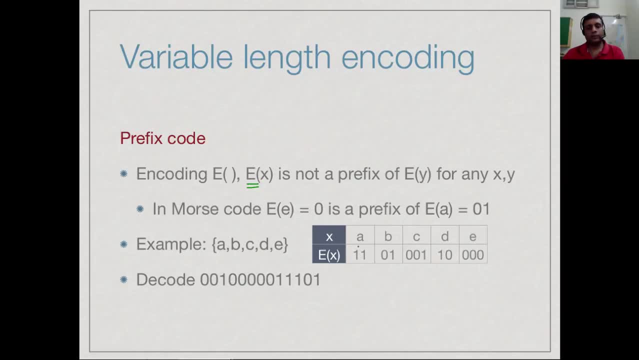 x is the encoding of the letter x. So here is an example. So we have 5 letters- a, b, c, d, e, and now you can check that none of these encodings can be extended to anything I do not have. if I see 1- 1, it must be an A. there is no other code which starts with 1- 1.. If 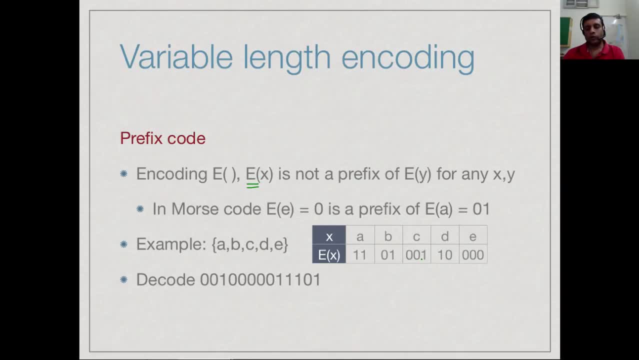 I see 0, 0, it is not a code, but 0, 0, 1 is a code, So 0, 1 cannot be extended, and so on. right, So each of these cannot be extended to be the code of any other letter. 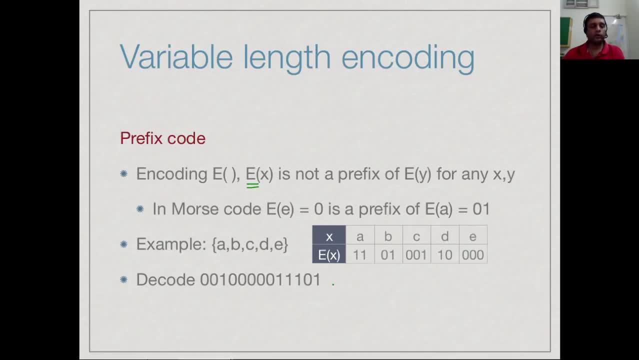 So now, when we get a long sequence like this, there is no doubt, right? The first point where I have completed a letter is 0, 0, 1, and this is a c. The next point where I have completed a letter is 3: 0s and it is an e. Then I read another c, and then an a, and then a b, right? 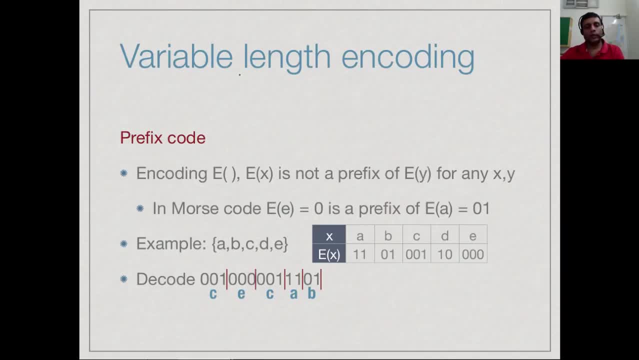 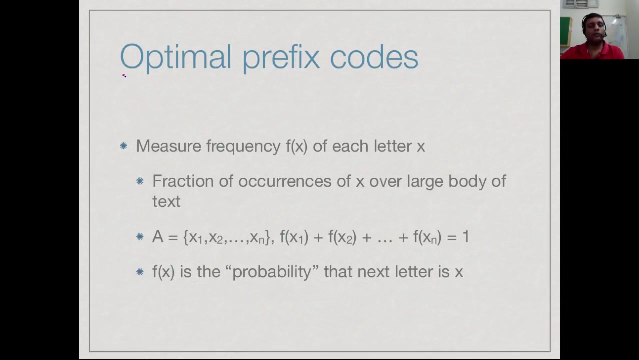 So if we have this prefix code property, that is, no letter is encoded to a string which is the prefix of the encoding of some other letter, then we have unambiguous decoding possible, and this is very important. So our goal is to find optimal prefix codes. So we need to talk about what we mean by 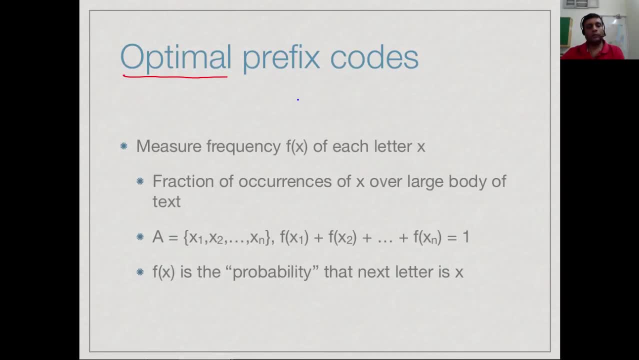 optimality. So remember we said that our goal is to assign shorter codes to more frequent letters. So somehow we have to determine what are more frequent and less frequent letters, right? So people have measured the frequency of the occurrence of each letter in different. 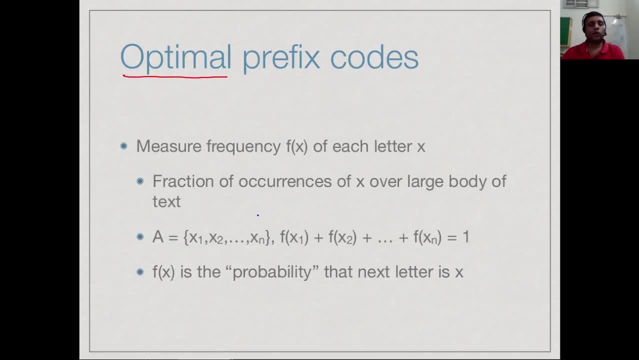 languages. So this is a very language specific thing, right? So this optimality- something which is optimal for English may not work for French. So you take a large body of text in a particular language, right- and then you count the number of a's, b's, c's, d's and e's and then you just look up the fraction out of the total. 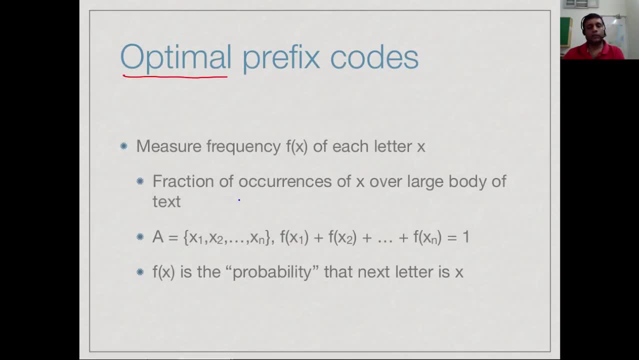 number of letters across all these text, how many are e's, how many are b's, how many are c's? So this is a kind of statistical estimate right of the average frequency of this. So this frequency will be a fraction. what? 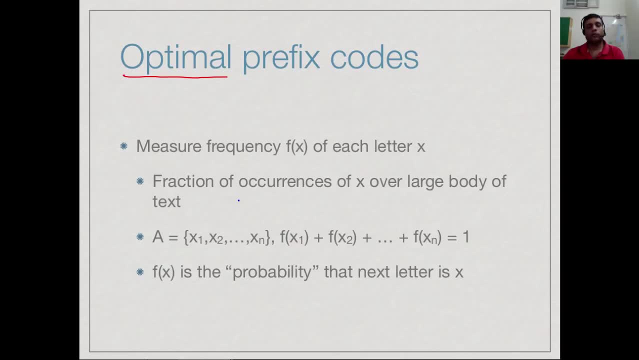 fraction of the letters over a large body of text will be e's. what fraction will be c's? And these, These fractions will add up to 1, right, because every letter must be one of them, right? So the fraction of a's plus the fraction of b's plus fraction of c's and so on is going to 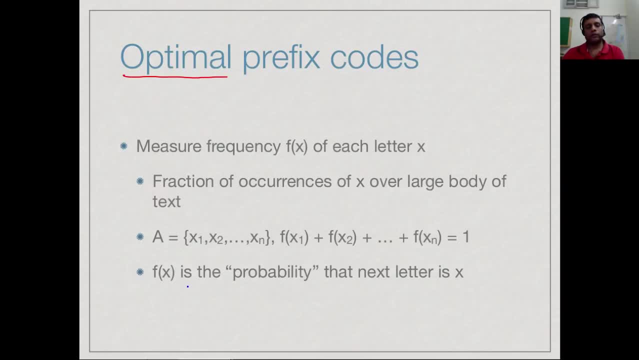 add up to 1.. And because of this, we can also think of this statistical estimate as a kind of probability, Like if I give you a random letter, if I look at a piece of text and I pick up a random letter from that text, what is the probability that is x. Well, it will. 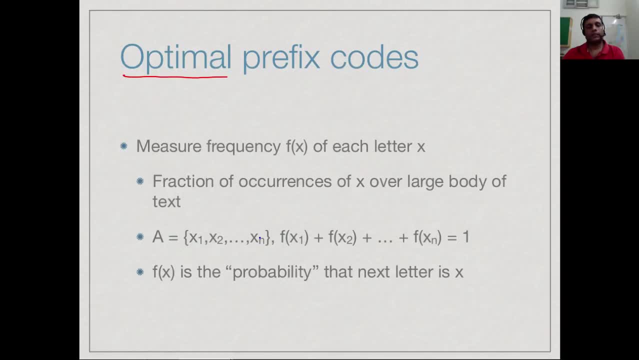 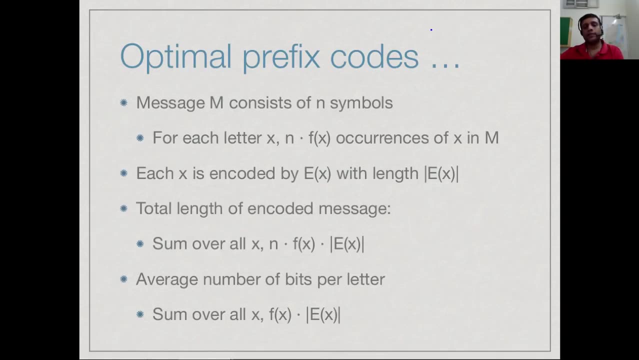 just be the frequency of x across all the text, right f of x, So these will add up to 1.. So now we have a message. it consists of some n symbols, right? So we have m 1, m 2 to m n, right? So these are my n symbols Now. 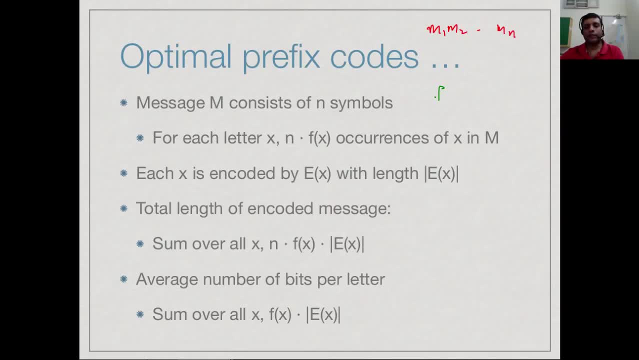 we know that if I pick a particular letter, x, then f, x fraction of these are x, right. So in other words, if I take n and I multiply it by the fraction, So say, if f, x is, say, one third, then one third of n, So n by 3 of these symbols will actually be the letter. x, right, And now each of these x's is going to be a fraction. So if I take n and I multiply it by the fraction, So say, if f x is, say, one third, then one third of n, So n by 3 of. 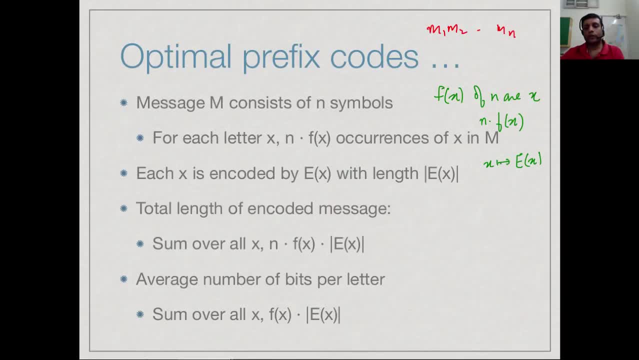 these is going to be represented by its encoding right. So supposing it is 0, 1, 0, then each x is going to be represented by 3 bits. So then n into f, x is the number of times I see. 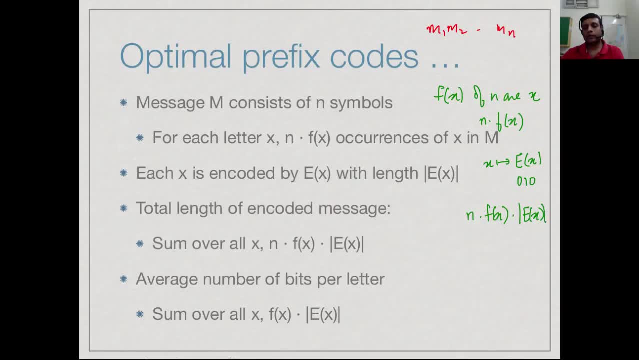 x, and this into the length of this encoding, is going to give me the total number of bits taken to encode all the x's in this message. Now, if I do this for every letter, ok, So if I take the summation over every y or every, 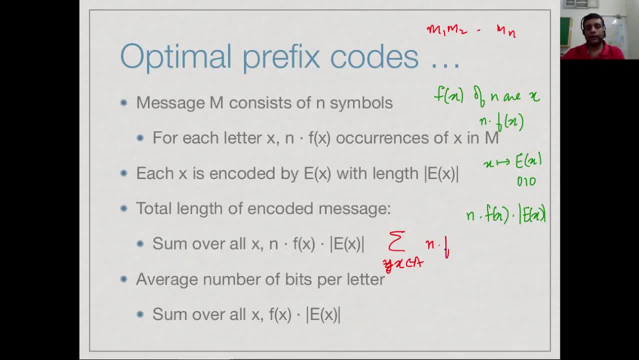 x in my alphabet, In my alphabet of n times the frequency of the letter, times the encoding length of that letter. ok, So this tells me how many bits I need to encode that particular letter. I add up all the letters, I will get the total length of the encoded message. right, And if? 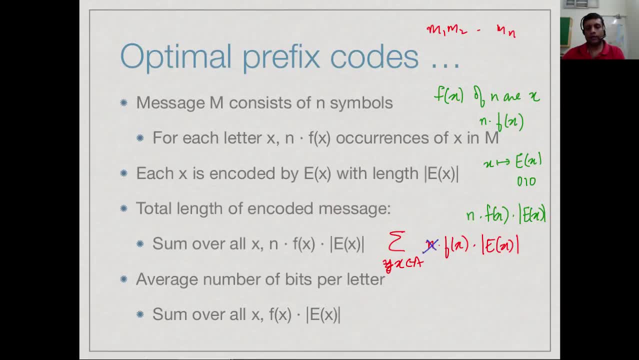 I do not include this n? ok, because notice that n is not a part of the summation independent thing, it is a fraction of any n, ok? So let us work out the total weighted average of the length of the encoding. So this is: 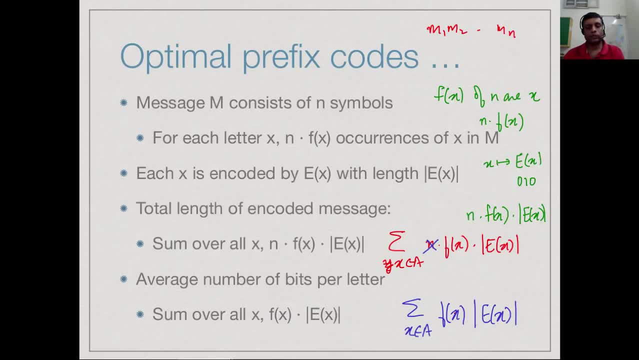 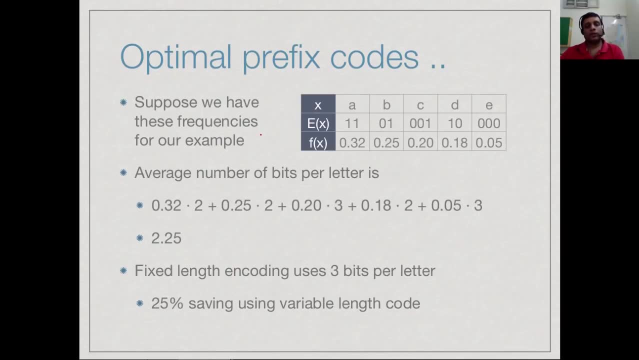 if you study probability theory, what is called the expected length of the encoding. So this is the average number of bits I use for the letter. ok, So let us work out how this. so suppose we take our earlier example on 5 letters now. 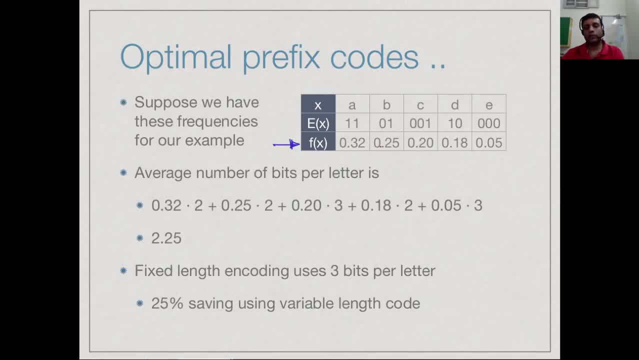 we insert some fictitious information about frequency. So this: all these 5 values are fraction in 0 and 1 and they all add up to 1.. Then if I do this summation over x of f of x, times the length of e of x, then I have: 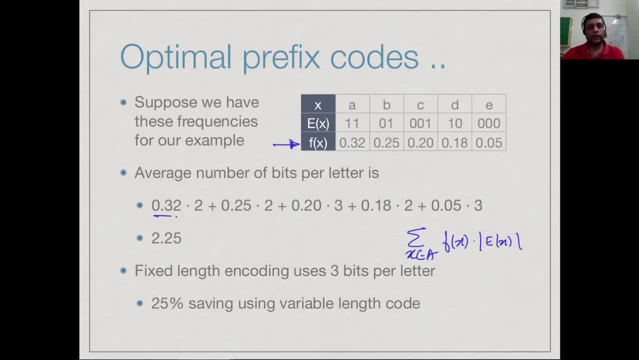 0.32 times 2, because the encoding of a is 2 letters. then I have 0.25 times 2, because the encoding of b is 2 letters, and so on. so I have these 5 terms: a, b, c, d, e, and then 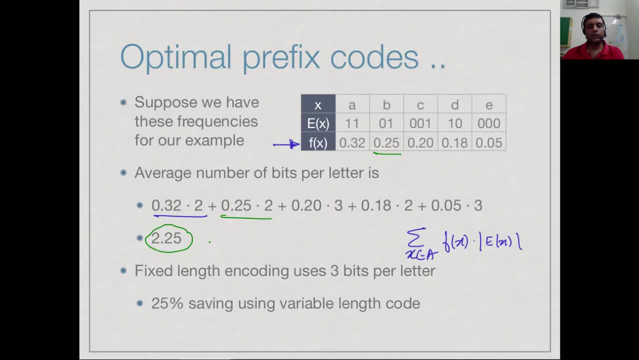 I add it up and I get 2.25. ok, So it says that I need, on an average, 2.25 bits per letter. of course I do not use 0.25 bits per letter, but what this says is, for instance, that if I have a 100 letters, I would 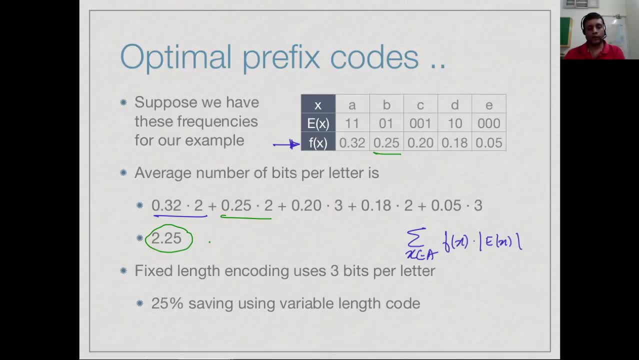 expect to see 225 bits in the output encoding. Now, a very specific kind of prefix code is the fixed length code, where, just by the fact that every code is of a fixed length, I know exactly where each one. So supposing I use 3 bits in this case, 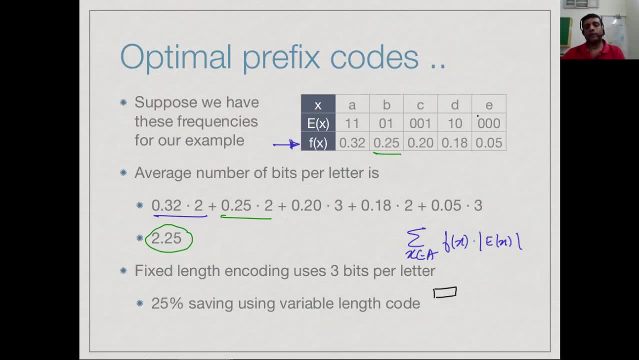 If I want a fixed length code of this, then there are 5 letters. so I cannot do it with 2 bits because I will only get 4 different combinations, so I need 3 bits. So if I use some 3 bit code, ok, then every 3 bits will be 1 letter, ok. 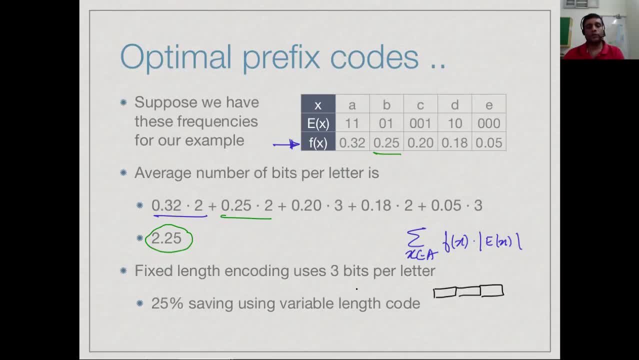 So in the fixed length encoding of this, I will use 3 bits per letter. so therefore, clearly, the number of bits per letter is 3, because I am using 3 for every one of them. And so by going to a variable length code encoding which takes into account the frequencies, 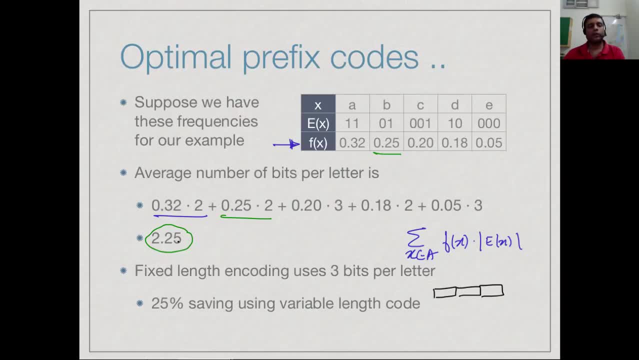 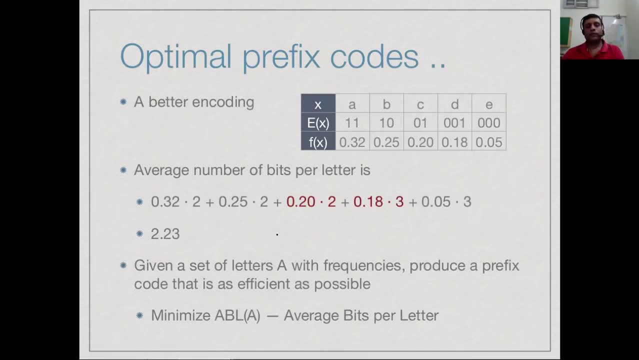 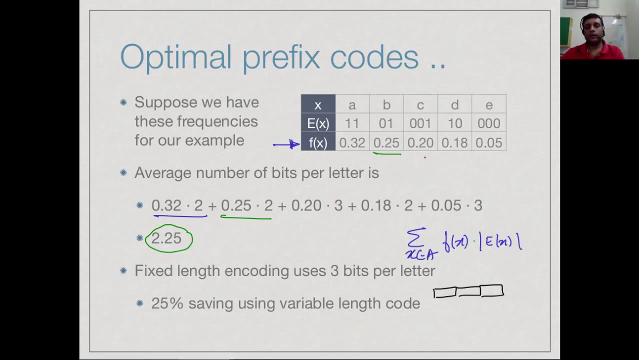 I am actually saving. instead of sending 300 bits for 100 characters, I am sending it to 25 bits, So you have a 25 percent saving. So this is what we are trying to get at. So in this example, in the previous thing, we had 2 frequencies: 0.2 and 0.18.. 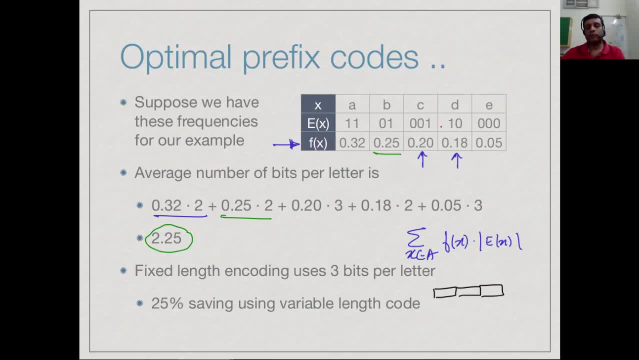 So 0.18 means d is less frequent than c, but somehow we had assigned c to be a longer code, So this violated our basic principle that shorter code should be assigned to more frequent letters. So if I see a pair of letters which are shorter than 0.18, then I can get 0.18. 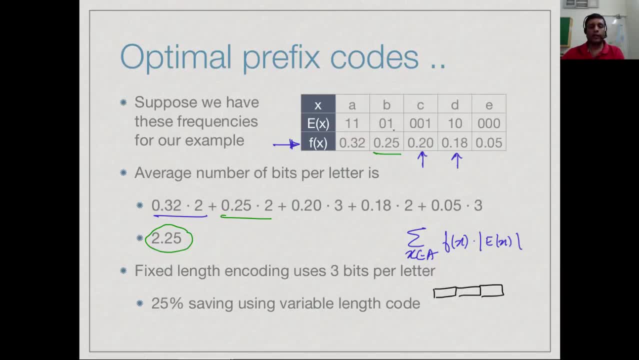 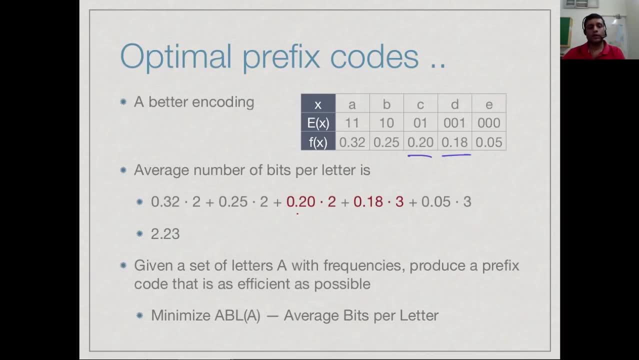 So this is what we are trying to get at, Where one is more frequent than the other. I expected to get a shorter code and I had not done so. So if I invert that, so supposing I now assign a 3 letter code to d and a 2 letter code to- 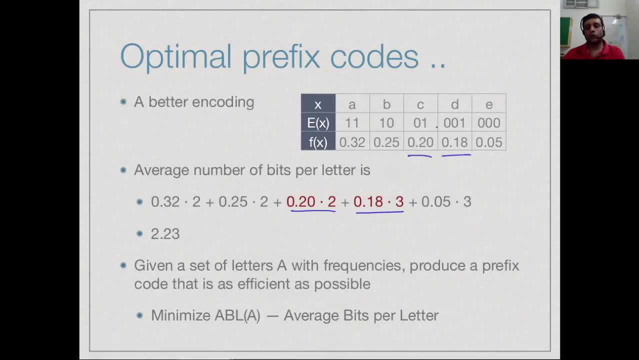 c, then these 2 terms change. the other terms, though the encoding may have deferred, the lengths, do not change. So then I get: instead of 2.25, I get down to 2.23.. So what this says is that, looking at different encodings, I could get different abl values. 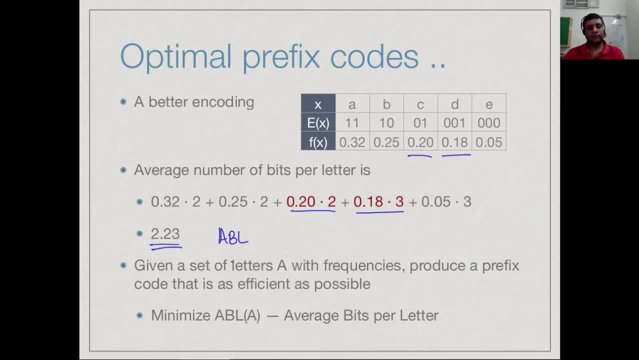 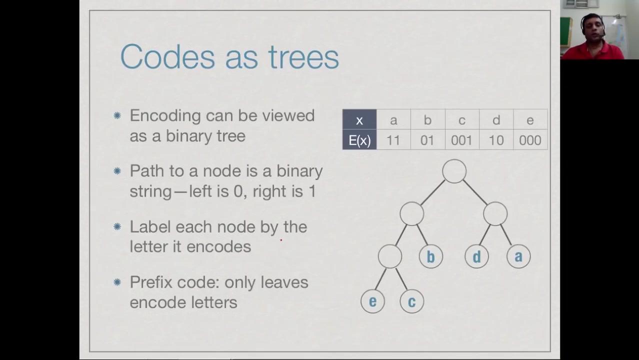 right 2.25, which would average bits per letter. So now our goal is to find an assignment capital E, which minimizes this quantity, so that our coding is as efficient as possible. So to get to this, it is useful to think of these encodings as binary trees. 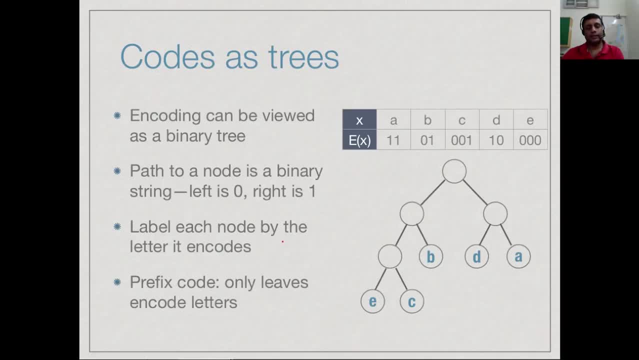 So in a binary tree I can interpret directions as 0 and 1.. So typically left is 0 and right is 1.. So now, if I read off a path in a binary tree, I am able tozuk an array like this one. So I focus on the length and width. I am able to even interest different trees that are on their grid. So when I enter the vector into binary tree, this goes towards this line- I am able to maintain the position or set the identity of the tree. 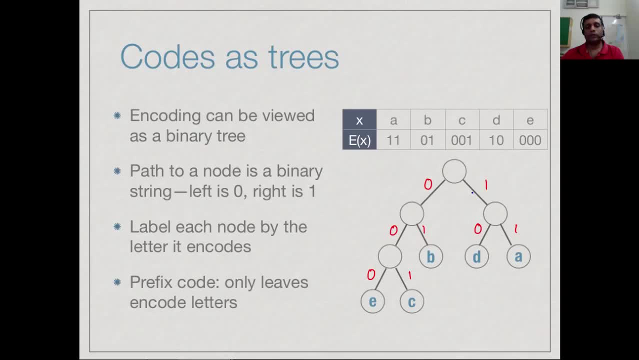 binary tree. it is also a binary sequence. So this path is 1: 1 on the right, for example, and this path, for example, is 0: 1 and this path is 0, 0, 0.. Now, if I read off a path and 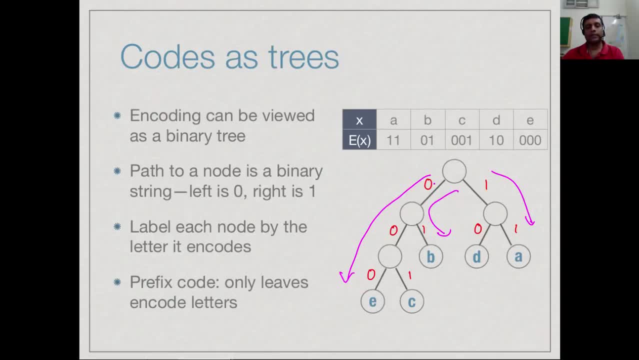 then I find a letter at that label, then it is as good as saying: is that that path labels that letter? that letter is encoded by that path. So here, because E is has the encoding 0 0 0 in the binary tree, I will follow the path 0 0 0 and label that corresponding letter. 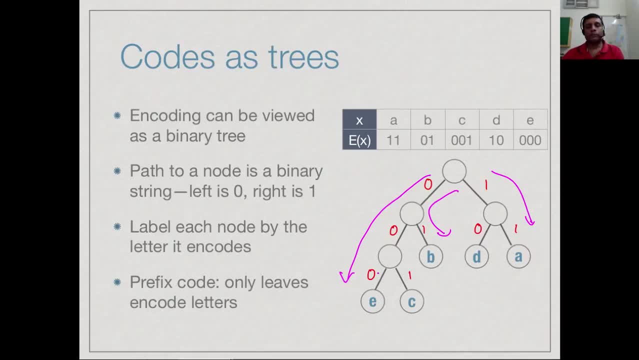 that vertex by E Now, because it is a prefix code. if 0, 0, 0 labels E, there will not be any code which says 0, 0, 0 and something more. there will not be another label below it. So these: 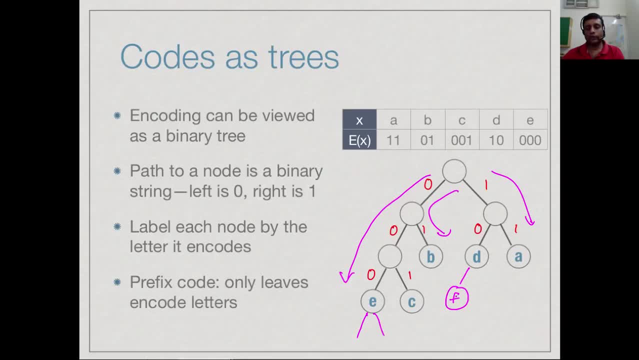 labels will not extend to other labels. I will not find an F below D, because otherwise it is not a prefix code. I do 1, 0 and I get a D, but I do 1, 0, something else and I get an F. So the prefix code for F extends the code for D. this is not allowed. So in a prefix 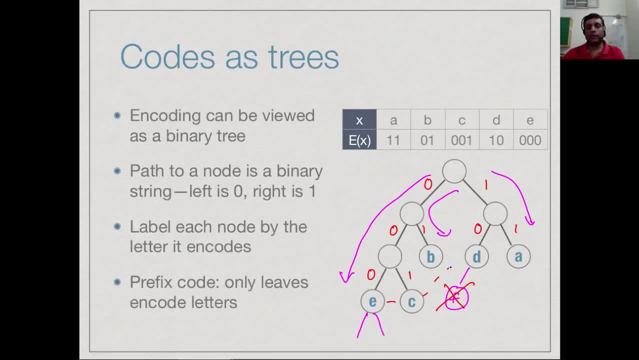 code. this cannot happen. So therefore all the labels are actually at leaf nodes. they are at nodes which have no successes. So here is an encoding for the other scheme that we had, where we exchanged the values of C and D. So now C has a 2 letter code and D 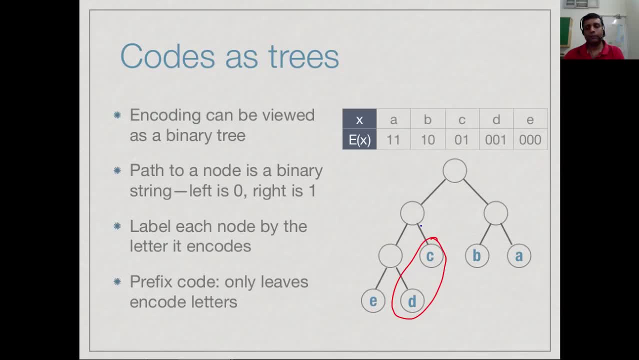 has a 3 letter code. So the depth, this is indicated by the depth. now the depth is the path. So the length of the path is the depth of the node. So C, in our earlier thing, was at depth 3 and now it is at depth 2, and likewise D was at depth 2 and now it is at depth 3.. 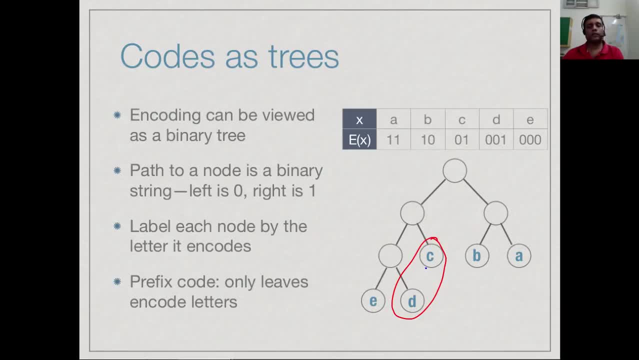 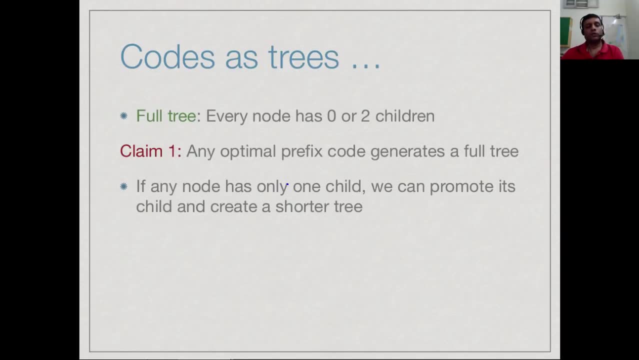 So we want to basically put things which have higher frequencies higher up in the tree at lesser depth. So, having encoded or looked at our encoding as a binary tree, we will now make a couple of observation, 3 observations about them, which will be useful to prove and 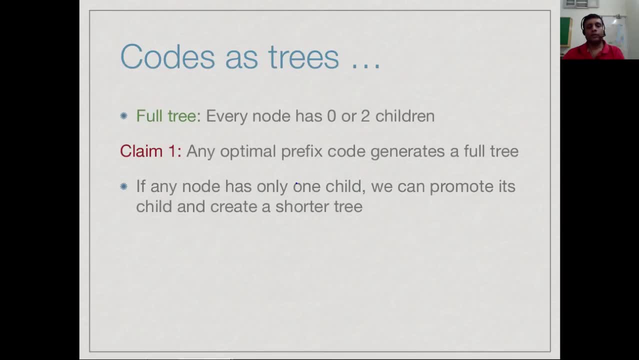 to develop an optimum algorithm and prove it is optimum. So the first thing is that in such a tree, if it is optimal, every node will either have no children, will be a leaf, or it will have 2 children. This is what you call a full tree. 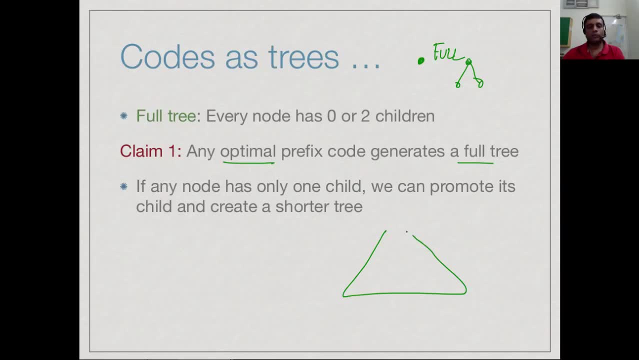 So every optimal tree is full. Now it is easy to see this because supposing we claim we have an optimal tree began a tree to the笑. discussion and goal count in our my project since 2015.. 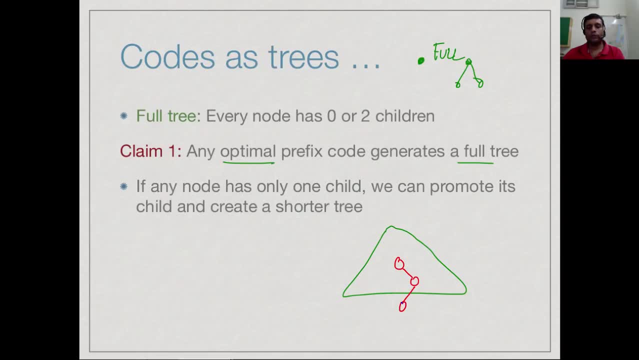 somewhere in between we had a node which had only one child. Then this child can effectively be promoted. we can remove this node completely and we can shrink the tree along this direction and nothing will change except that the depth of the nodes below it will become less So. 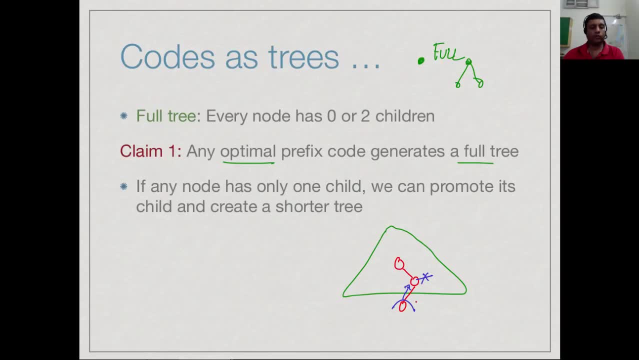 in fact we will possibly get a shorter average bit length than we had before, right. So therefore by having a singleton, either only a left child or a right child, we cannot be optimal. So every node must have either 0 or 2 children. 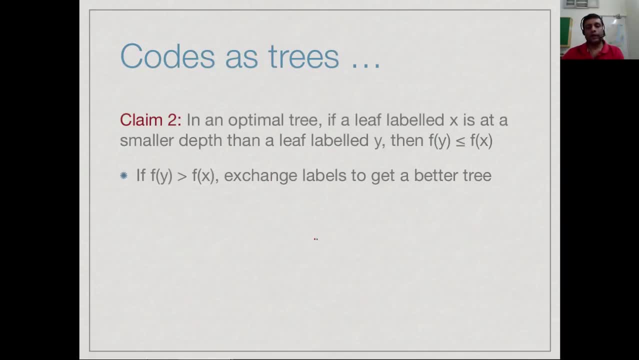 The next property is exactly what we saw in the earlier thing, which is that if I have two nodes, x and y, such that x is higher than y, So x is at some level and y is at a different level, Then x has a shorter encoding than y. this must mean that f of x is higher than. 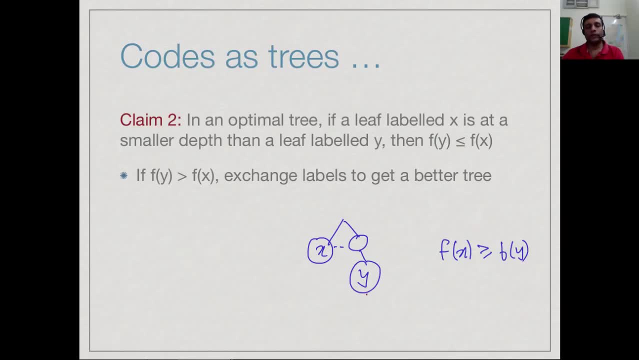 x at least as much as f of y. In other words, when I go down the tree my frequency cannot increase, because if f of y were bigger than f of x- that if I had more y than x is in my text, then I would just exchange these two right? I would find a better encoding by putting: 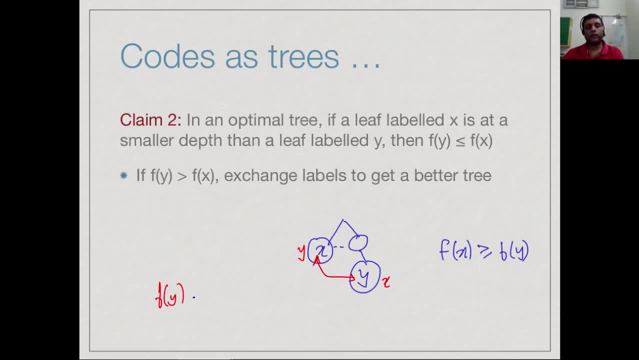 y here and x here. because now if I do f of y times the length of y or the depth of y in this tree, then it will reduce because the depth of y is reduced and this is a higher multiplier. So therefore, if I had a higher thing below, 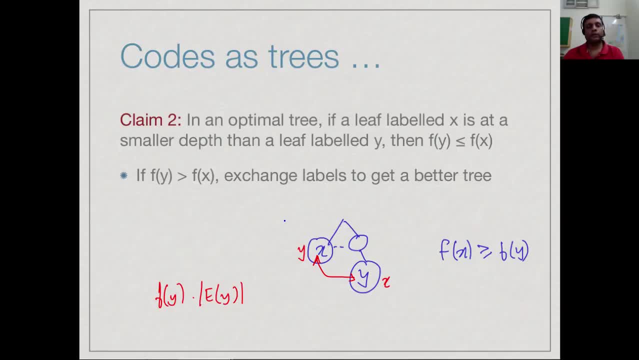 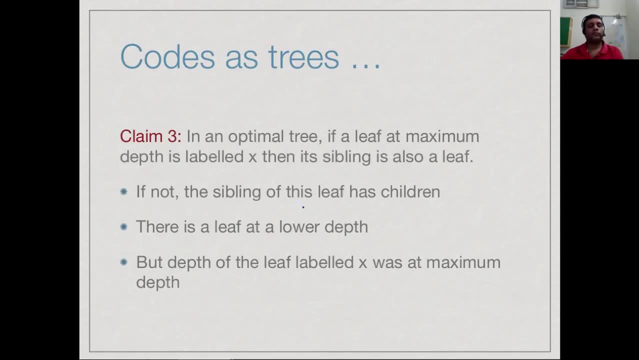 then I could exchange. that does not get a better tree, and that does not happen when an optimal tree, So then an optimal tree. if I go down the tree, I would only find lower frequency letters. The final property is to do with leaves at the lowest level. So supposing I have a leaf at the lowest level, right? So this is some. 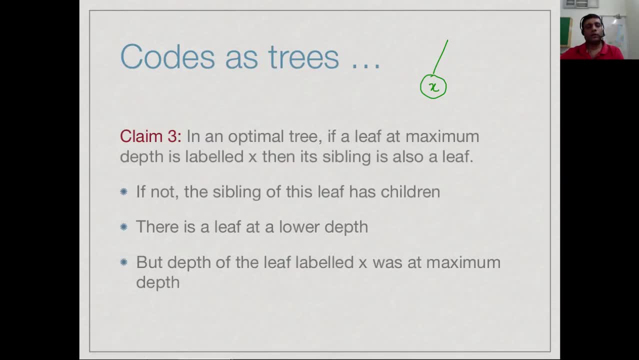 leaf at the lowest level. So I know, because it is an optimal tree, that it cannot be an isolated child. it must have a sibling, right? So I go up and come down, it must have a sibling. Now there are two possibilities, right? The two possibilities are: this is a leaf or the. 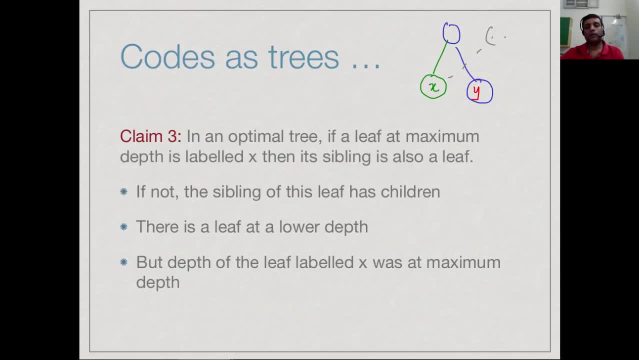 other possibility is that this is not a leaf right. The claim is that if it is not a leaf, then it must have children. So then there are leaves here which are at a lower level than x, but x is assumed to be a maximum depth leaf. ok, So a maximum depth leaf cannot have. 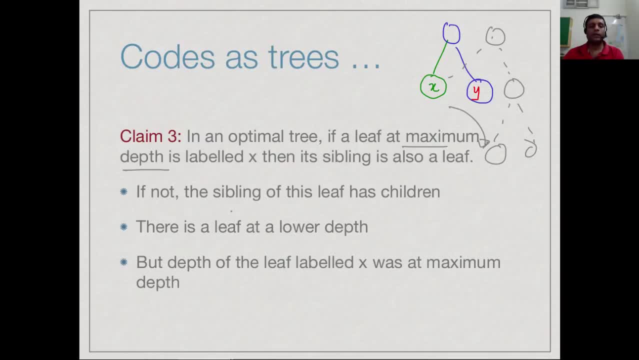 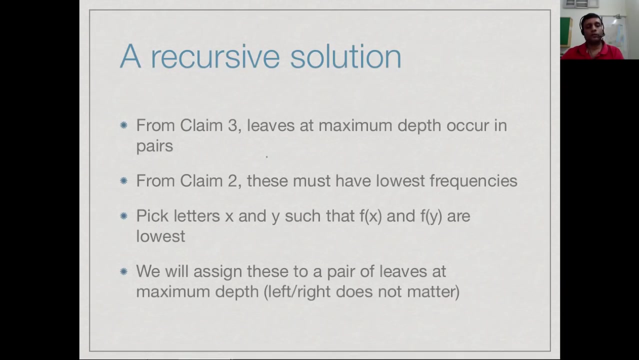 a sibling which is not a leaf, because its sibling would then have children which have a higher depth right. So therefore, if I have a maximum depth leaf in my optimal tree, then it will occur as a pair with another maximum depth leaf right. So this is a conclusion that leaves at maximum depth occur in pairs, and then we know that. 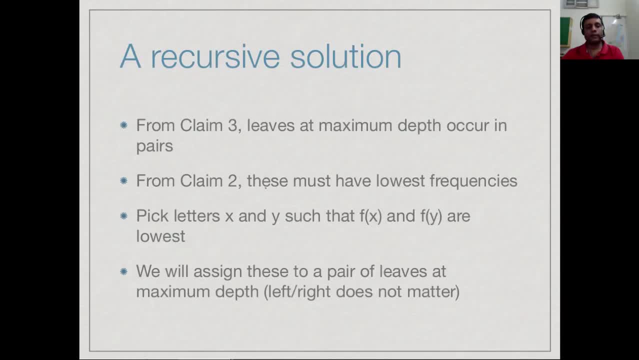 because the frequencies keep dropping as we go down, increasing in depth, So these pairs must have the lowest frequencies among the lowest frequencies. So now, in order to develop the solution, we will use recursion. So what we will do is we will say: let us. 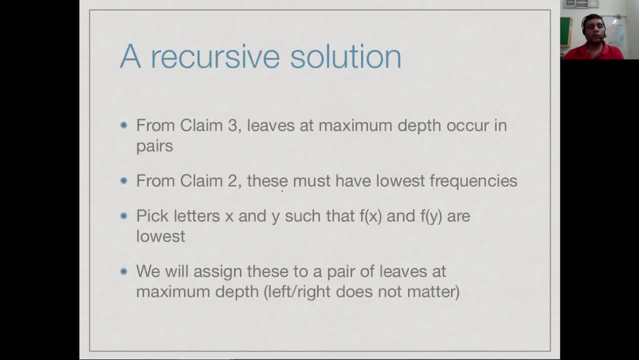 look in the overall table that we start with and pick two letters which have the lowest frequency, So we can assign them the longest codes, So they can be put at the lowest level. and then we know that the lowest level leaves occur in pairs. So let us assume that these 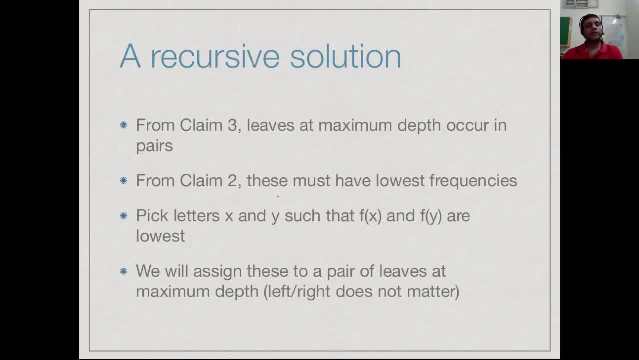 will be paired out. ok, So we will assign these lowest frequency letters, x and y, to a pair of leaves at the maximum depth. left and right does not matter, because it is only the depth that matters. So now the recursive solution will say that: 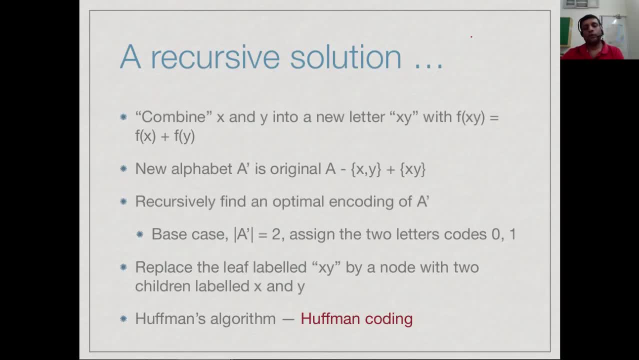 ok, how do I figure out what the rest of the tree looks like? Well, if I have a situation where I have decided that x and y go here, ok, then I will kind of treat this as a unit and make a new letter called x- y and give it the cumulative frequency f? x plus f? y of 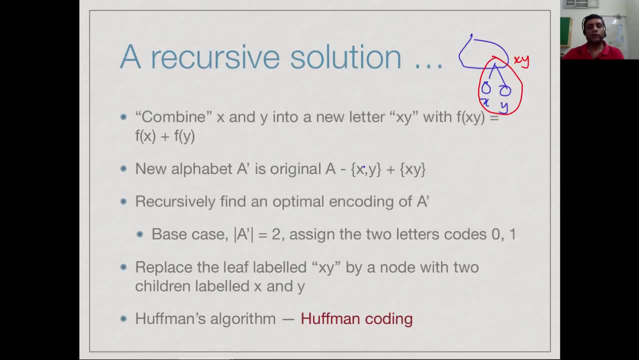 the old two letters. So I will construct a new alphabet in which I drop x and y and I add a new composite or hybrid letter, x, y, whose frequency is going to be f x plus f y. Now recursion kicks in. I have a k minus 1 letter alphabet, ok, So I will recursively find an optimal encoding. 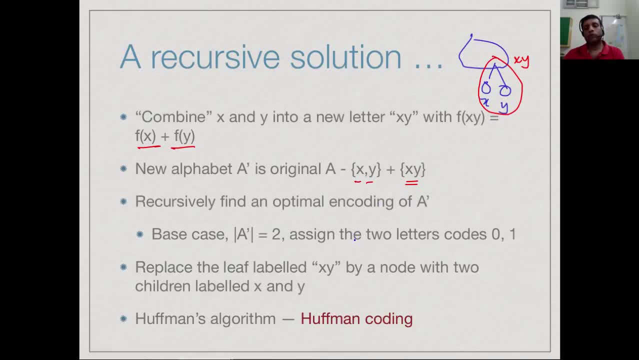 of that. Now, before coming to how to adapt the solution, the recursion ends when we have only two letters. For two letters, the optimal solution is to build a tree which has exactly two leaves labeled 0 and 1 as the path. ok, So this is. 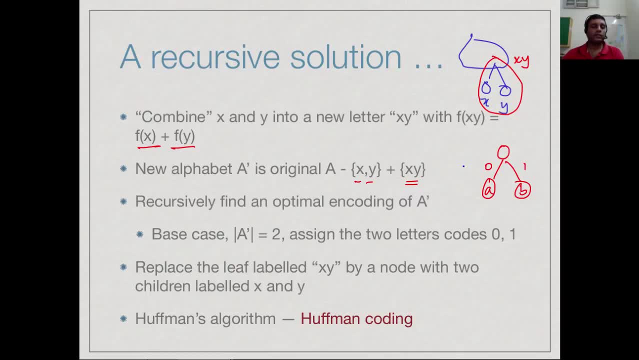 the base case. So if I have more than two letters, I will recursively construct a tree for the smaller thing and then I will come back. and now in the tree that I constructed I will have somewhere a leaf labeled x y. Now, x y is not a letter, So what I will. 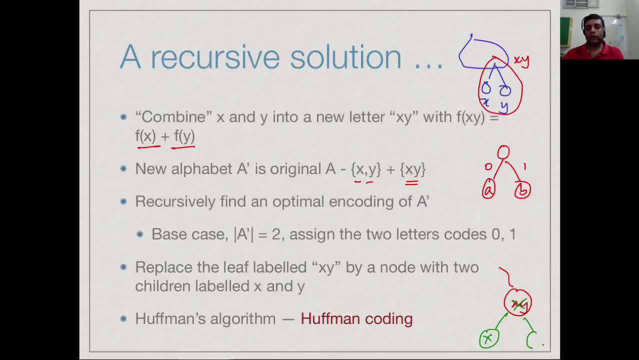 do is I will replace this by two new leaves called x and y, So I will go from the tree over a prime to a tree over a by doing this. ok, So this is an algorithm called by, double, developed by Huffman, and this type of coating is called Huffman coating. 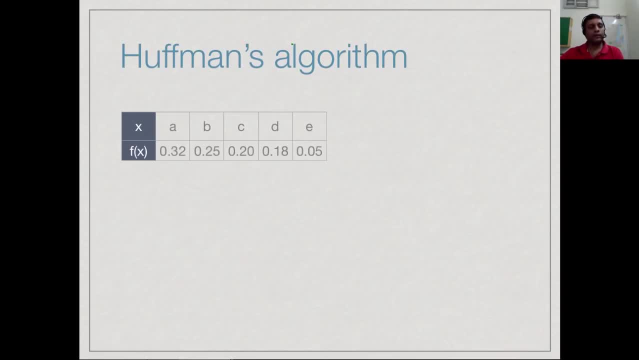 So let us look at this example that we had earlier. So here the two lowest frequency letters are D and E, So we merge them into a new letter: D, E, and this is a frequency 0.23, because it is 0.18 plus 0.05.. Now these two are our two lowest letters, So we merge them. 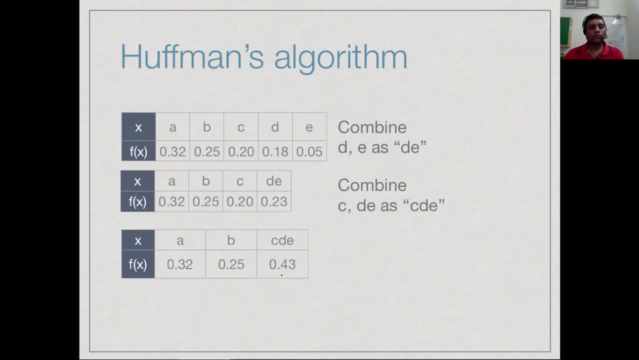 and we get a new letter C, D, E of cumulative frequency 0.43, which is the sum of all the frequencies of the components. Now it turns out that these two are the smaller two, So I merge them into a letter A, B and now I have reached my base case, where I have exactly 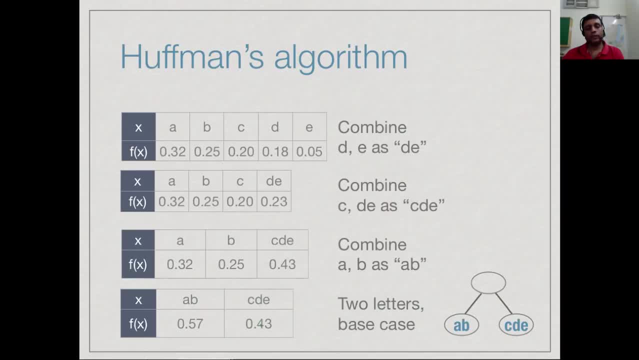 two letters, So I can set up a trivial tree for these two letters labeled 0 and 1.. And now I work backwards, So the last thing I did was to merge A and B. So now I will take this A- B thing and split it up. So I will take this A- B thing and split it up, So I 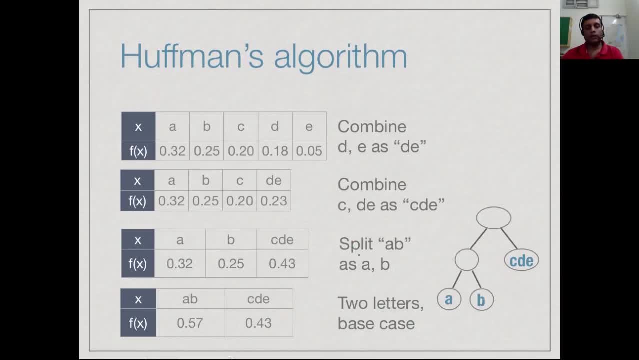 will split it up as A and B. So I will split A, B as A and B and I will get this tree Then. the previous step was to combine C, D, E into C and D. So I am going to split this up as. 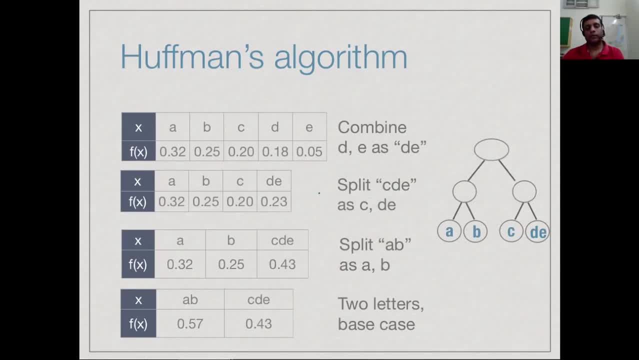 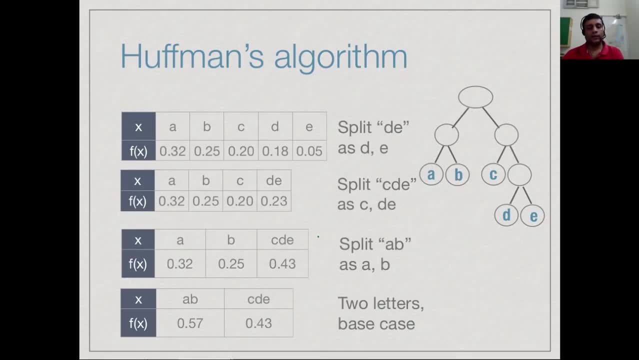 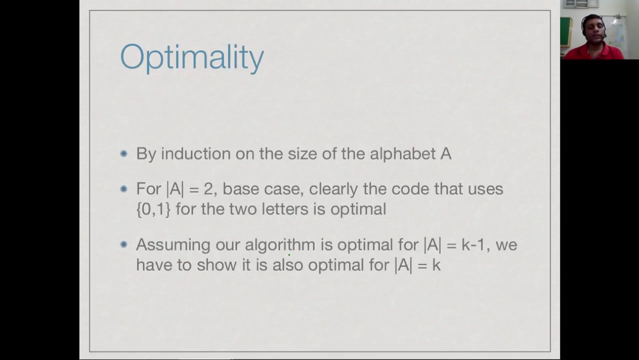 C and D And finally I am going to split this up as D and E. So this is how Huffman's algorithm works, by recursively combining the two lowest frequency nodes and then taking the composite node and splitting them back afterwards. So to show that this algorithm is optimal, we will go by induction on the size of the. 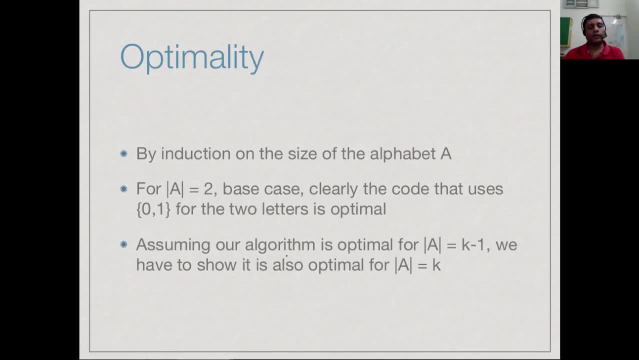 alphabet. Now, clearly, when I have only two letters, I cannot do any better than assign one of them 0 and one of them 1.. So the base case is optimal. So we will assume that this is optimal for k minus 1 letters and now show that it is also optimal for k letters. So 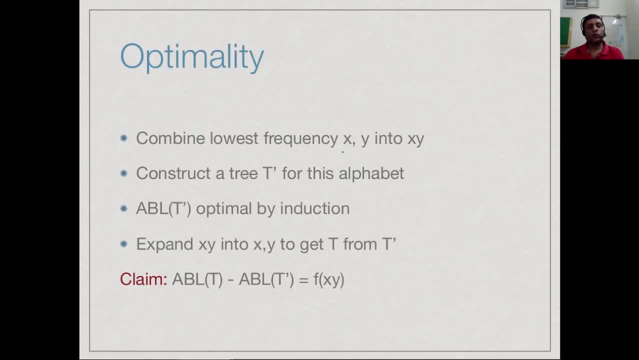 recall that we went from k to k minus 1 by combining the two lowest frequency letters as one, constructing an optimal tree for this tree. So this is the optimal tree for this lower, smaller alphabet, and then expanding the x, y to get a new tree. So the claim is: 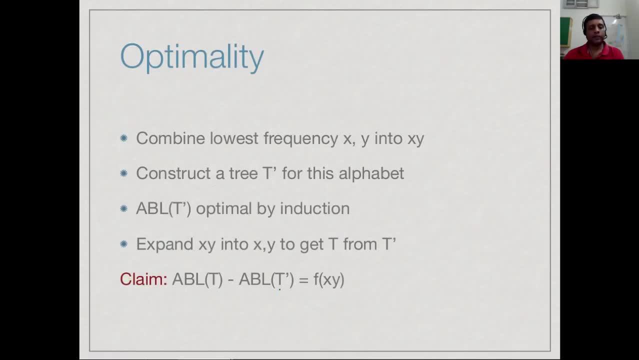 that when I go from the tree over k minus 1 letters to the tree over k letters the cost is going to increase. but this cost is going to be fixed by whichever letters I chose to contract. So if I chose x and y to merge, to go from t to t prime, then the amount by 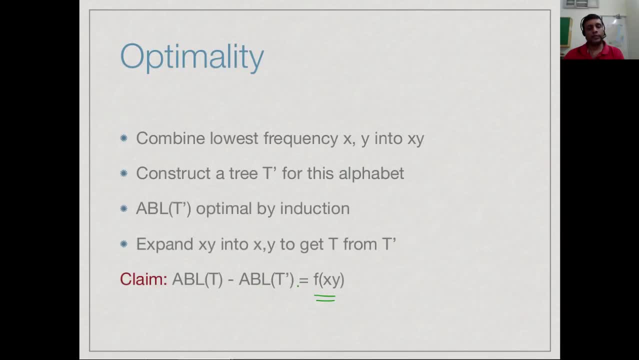 which the average bits per letter is going to change is exactly the frequency of this combined letter f, x, y. So it is deterministically fixed by which one I chose. So even though I do not know the cost of the trees directly, I can tell you that the cost is going to be different. 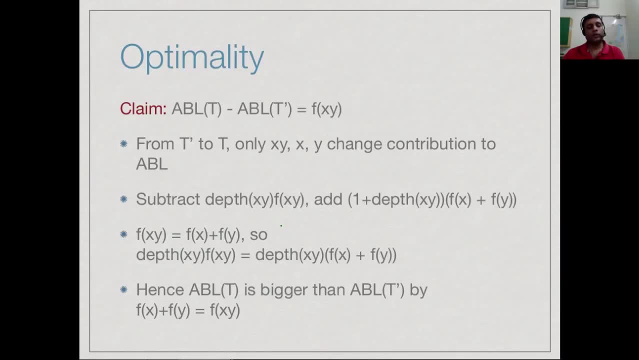 by this amount. This is not very difficult to prove. So in that summation that we had, so in the tree notation, remember, this depth of z is the same as the length of the encoding. So the depth exactly reflects the length of the string used to encode it. So this is: 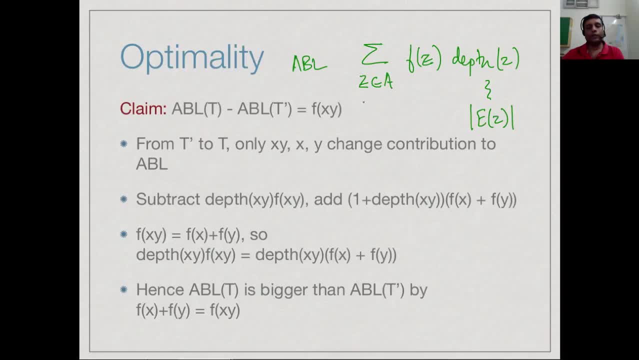 our abl calculation. Now, for every node other than x, y and x y, they are exactly in the same position in t and t prime. So this summation, the terms do not change. So the only changes are between these three nodes. So what I will do when going from t prime to t is I: 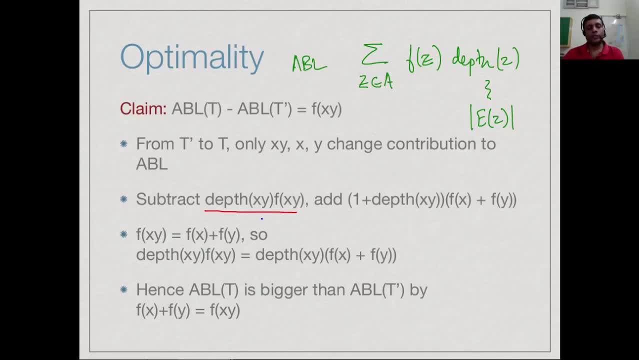 will remove this contribution of the composite letter x- y And then, at the next level, which is 1 plus the depth of the x y, I will add the node f x and I will add node f y. So I will get the combination of the x y, f x times that plus f y times that. So I am subtracting. 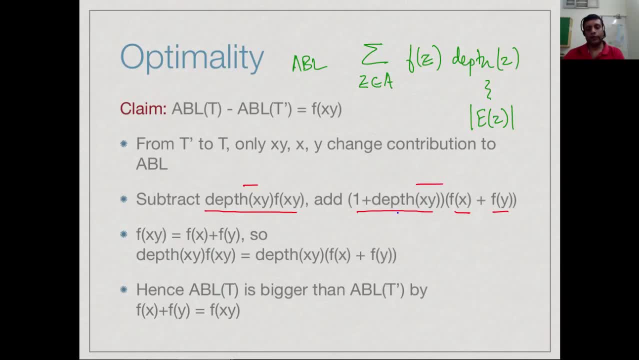 this amount on the left, then I am adding this amount on the left. So now actually f of x y is nothing but f x plus f y. So this left hand side term is actually this right hand side component: depth of x y. 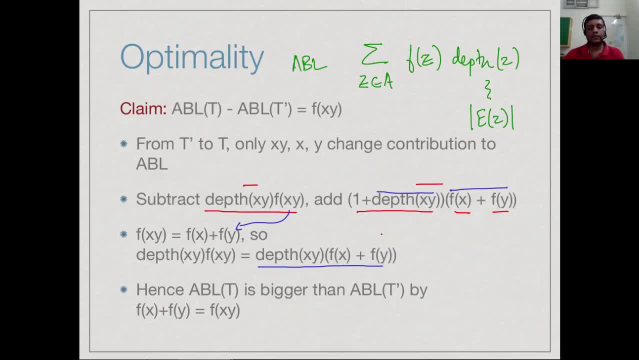 f x plus f y times f x plus f y. So I am subtracting this and adding it back, so they cancel each other out, ok? So therefore, all I am left with is 1 times f x plus f y, which is f x plus f y or f x y, right? So therefore, in going from t prime to t, the crucial thing- 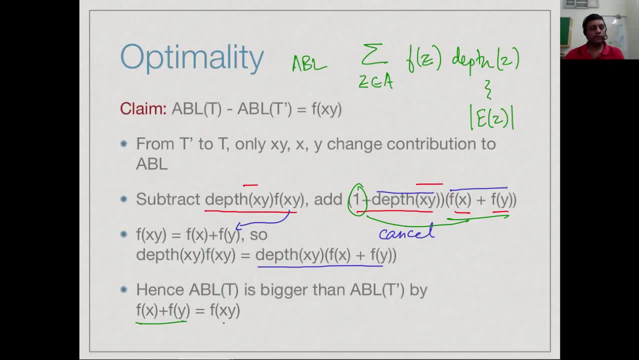 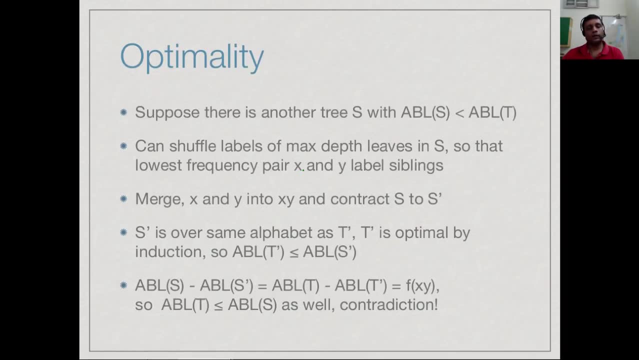 is. it only depends on which letters I contract. that fixes the difference uniquely. Now let us assume that we know how to solve all k minus 1 size alphabets efficiently and we have done this recursive thing to construct the tree t for size k, Suppose there is another. 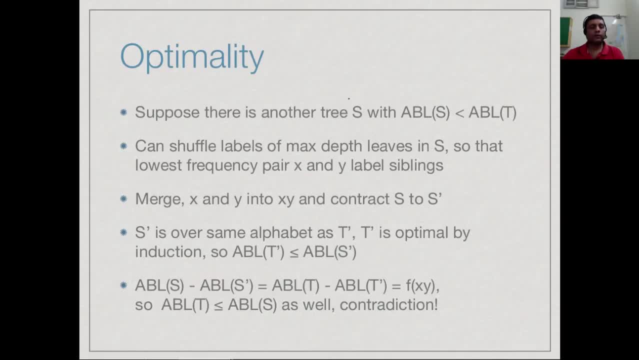 strategy which produces a better tree for size k. ok, So there is another tree, candidate tree S produced by some different strategy whose average bits per letter is strictly better than the one that we construct recursively Now in S. we know for sure that the average 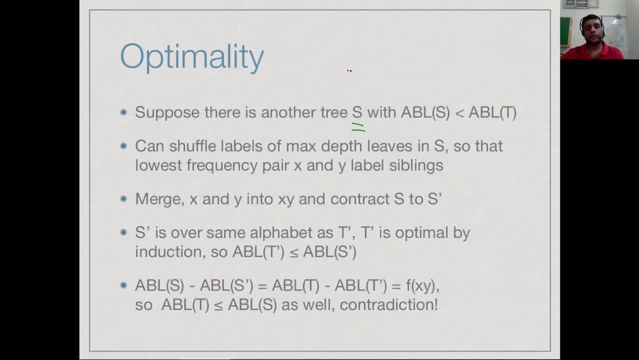 bits per letter that we use in the recursive construction: x and y. ok, So they occur somewhere at the bottom of this tree. ok, So this is my tree S. ok, So these must be leaf nodes because they have the lowest frequencies over all the letters, So they must be at maximum. 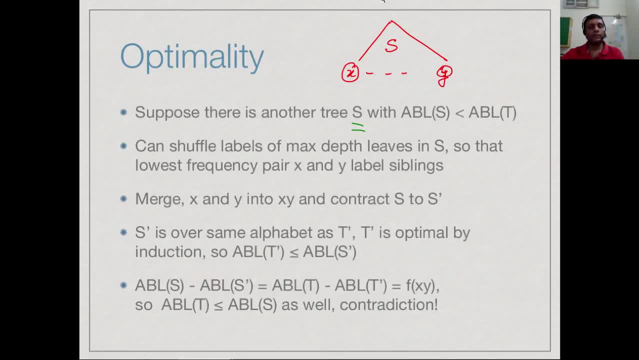 depth, but they may not be next to each other, but it does not matter, because since they are both at maximum depth, I can move them around. at this depth. I can move letters around, I can reassign them to other leaves at the same time. 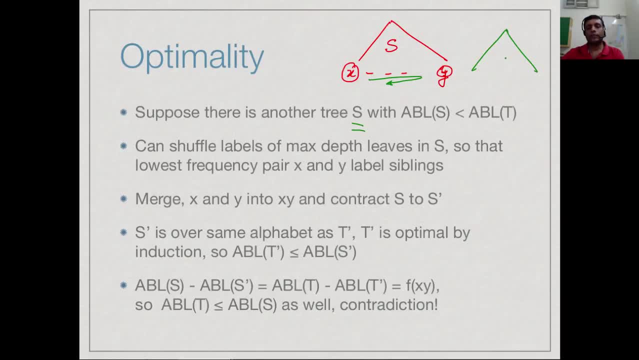 So that is that I come with the configuration. I come to a new S- I call it S again- where I actually have x and y together. ok, So I can assume that the S that has this optimal property, which is better than the tree I construct, it actually has x and y as sibling leaves. 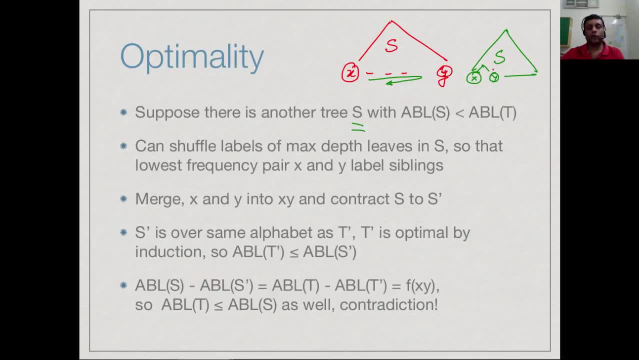 at that maximum depth. Now what I am going to do is, in this S, I am going to concretely fuse this and get an S prime. So this S prime will be over. So this S prime will be over k minus 1 letters, except, instead of doing it by a recursive call, I am actually taking 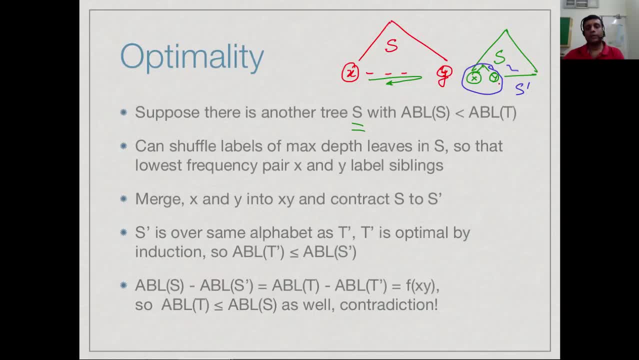 a concrete tree over k letters, and I am actually compressing two nodes into one and calling it a tree over k minus 1 letters. But because this is over k minus 1 letters and this represents an encoding, ok, It cannot be any better than the encoding that I recursively computed for. 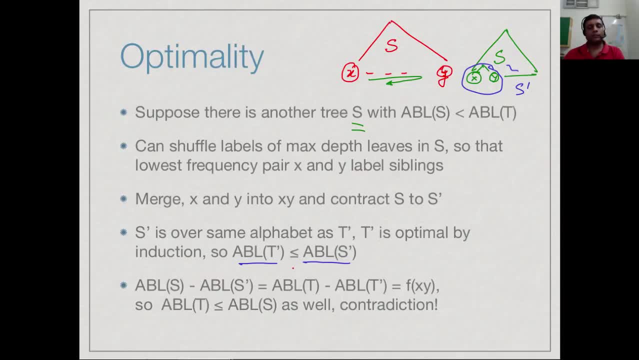 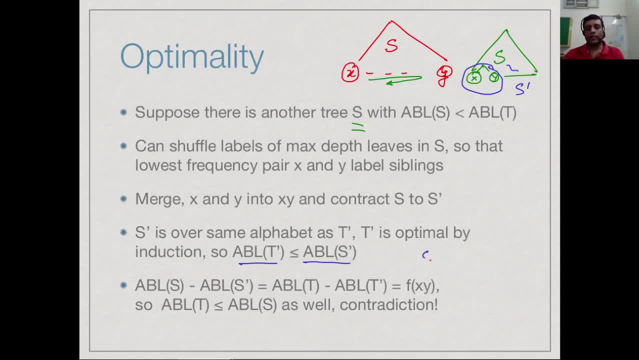 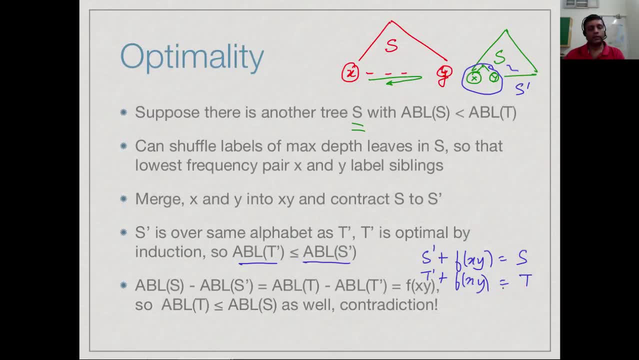 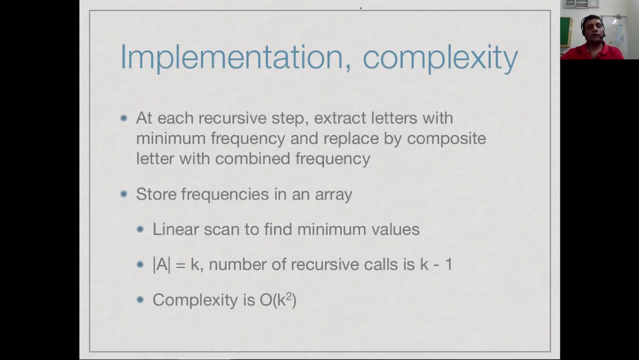 T prime, then S cannot be any better than T. So it was a contradiction to assume that S was strictly better than T. So this proves that our strategy of recursively computing T is optimal for all k. A word about the implementation. ok, So what we have to do is k minus 1 times. we have to 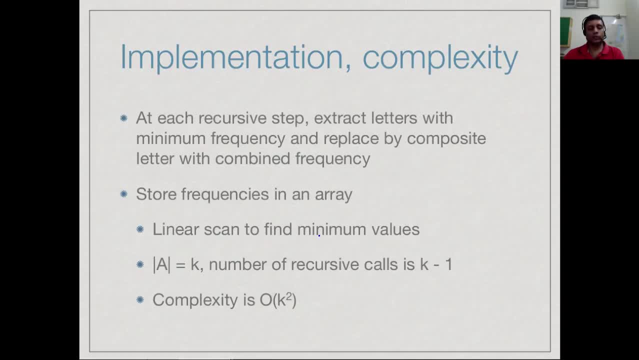 merge these two minimum values and compute a recursive solution right. So the bottleneck is finding these minimum values. If we use an array, then, as we know, we will have to scan the array each time to find the minimum values. Remember that the minimum values keep changing. 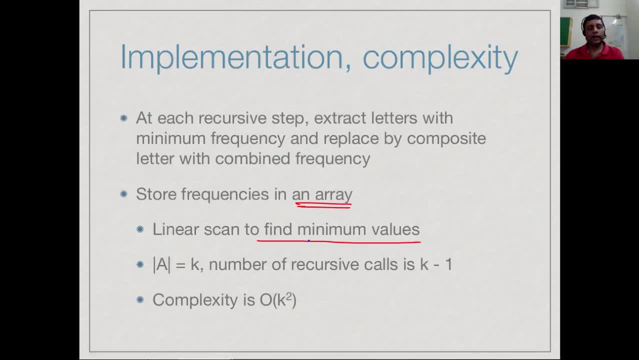 I cannot sort it once and for all, because each time I combine two letters, I introduce a new letter into my array with a new minimum value which was not there before, but not a new value which is not there before, which may or may not be the minimum. 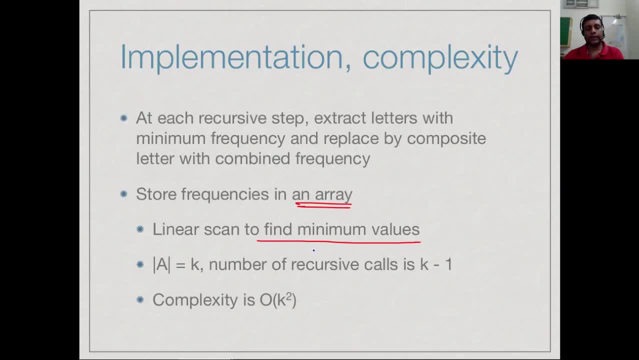 So at each stage I have to find the minimum. so it is an order k scan each time, right, so linear scan, and I do this about k times, So I get order k square. but it should be fairly clear to see that this bottleneck can be got around by using a heap. So that is precisely. 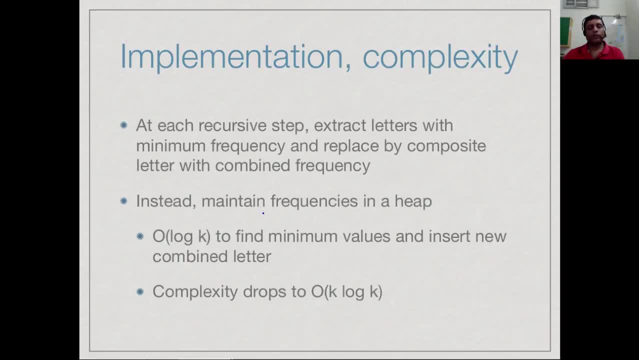 what heaps are good at finding the minimum right. So if I maintain the frequencies not as a simple list or array but as a heap, then in order log k time I can find the minimum values and then I can insert back the new composite letter also into the heap and log. 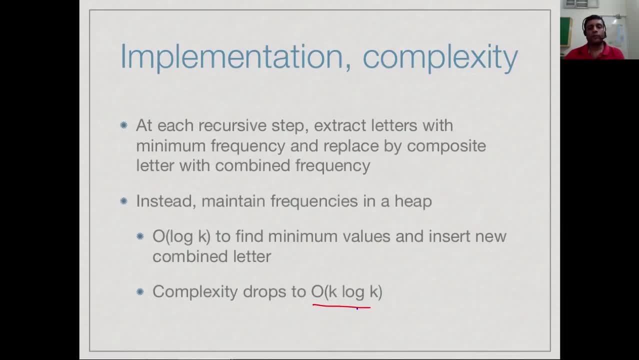 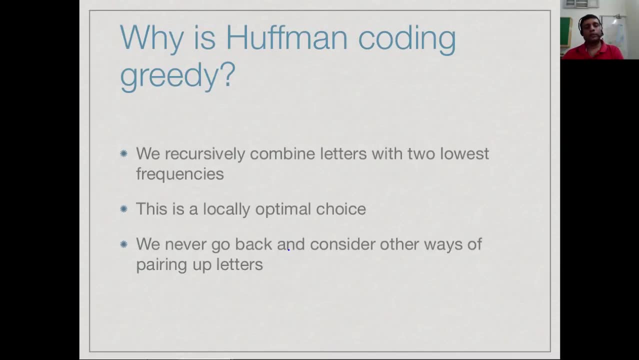 k time. So each iteration takes only log k, and so I improve from k square to k log k. So recall that we mentioned at the beginning that this is going to be our last greedy algorithm. So why is this greedy? Well, because every time we make a recursive call, we are deciding. 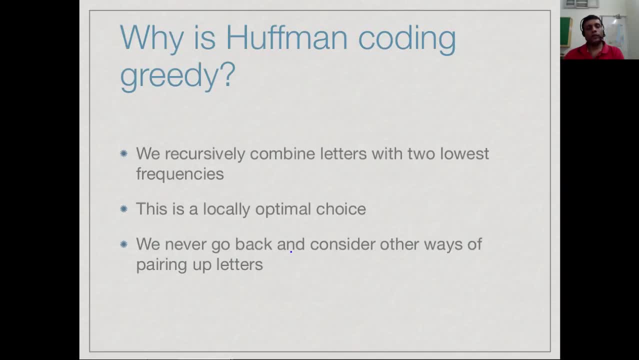 to combine two nodes into one, and the two letters we choose are always the ones with the lowest frequencies. Now, what is to say? that we could not do better by choosing the lowest and the third lowest? but we never try it. We only try the lowest and the second. 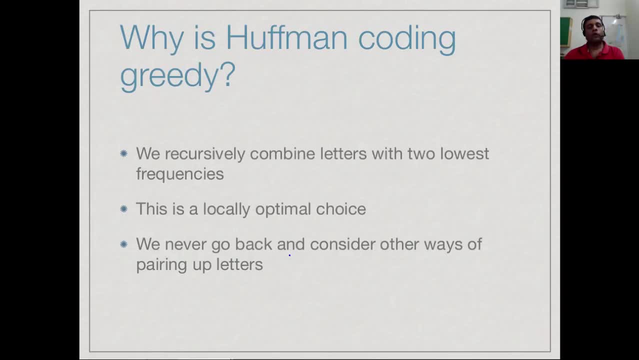 lowest. So we make a locally optimal choice and we keep going with this choice, never going back to revisit it, and finally we get a global solution. Now we have proved that this global solution is actually optimal, and we have to do that because there is no other reason to. 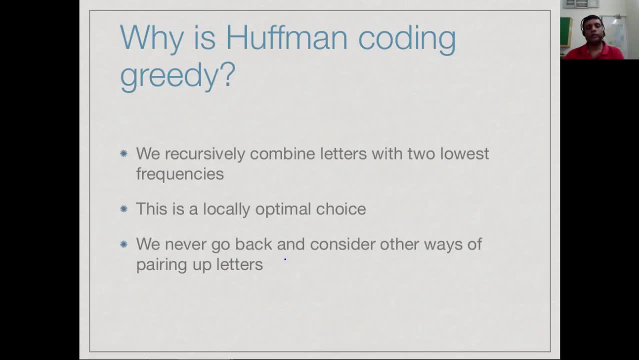 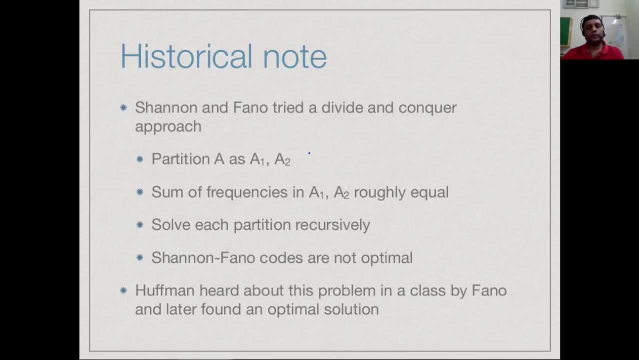 expect that by making this short sighted choice At the current time, take the two worst frequencies and combine them- that you are always going to get the best solution. So this is very much a greedy strategy. So finally, a brief historical note. So Claude Shannon is the father of information theory.